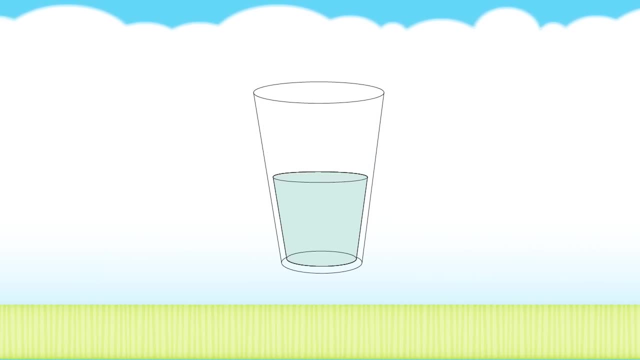 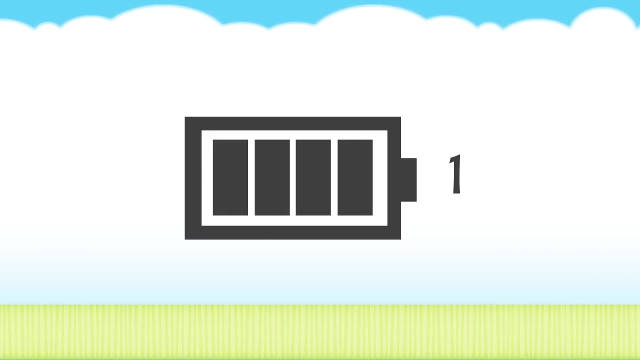 With a quick glance you know when a glass is full, half full or nearly empty. When you see a battery icon, you can tell whether it's completely charged, half charged or exactly a quarter, Because you know these things automatically. you can see for yourself. 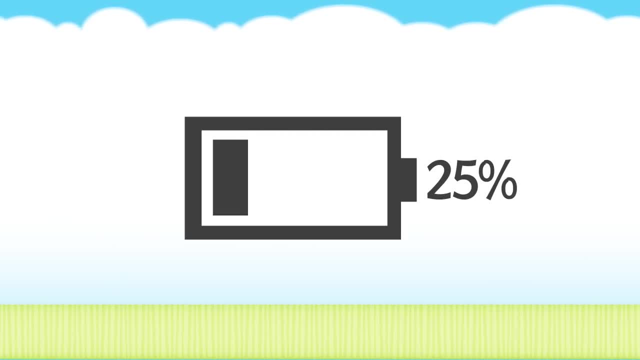 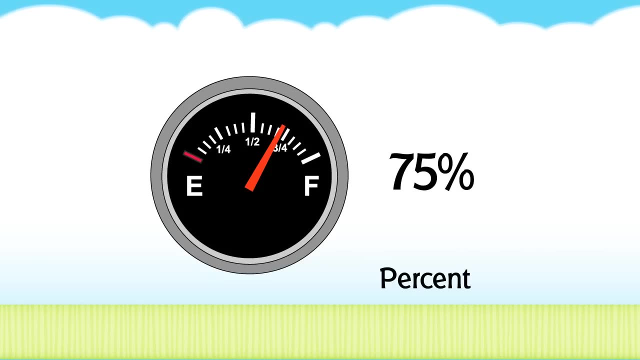 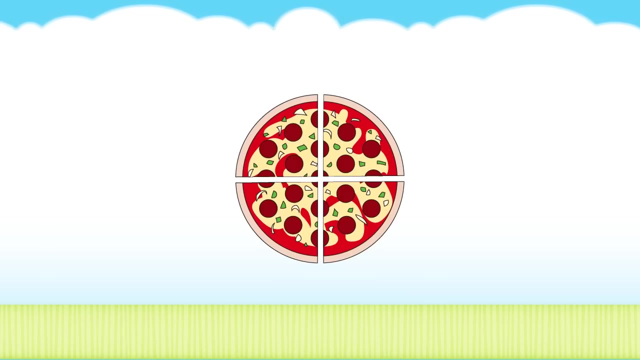 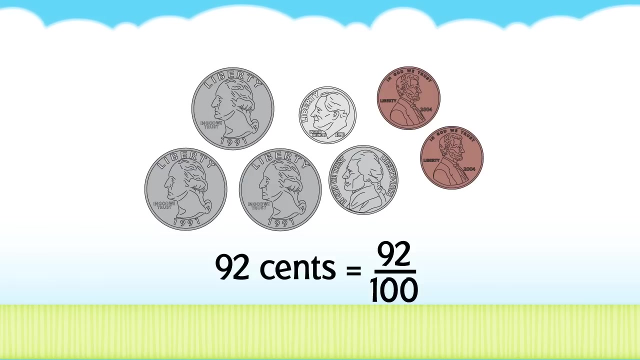 that decimals, fractions and percents give you different ways of stating the same information. You can show the parts of a pizza or the parts of a group. the same way. When you see any fraction, decimal or percent, remember that you can express it in two other ways. 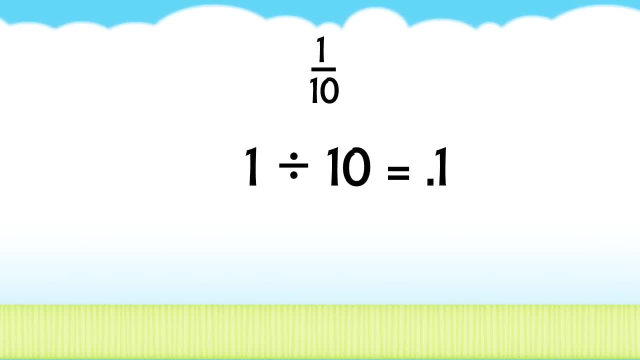 Practice converting fractions into decimals and decimals into percents. It's easy once you see how. Divide the numerator by the denominator, The numerator 4, divided by the denominator 8, equals 0.5, or 5 tenths. That shows you the decimal 0.5 times 100. 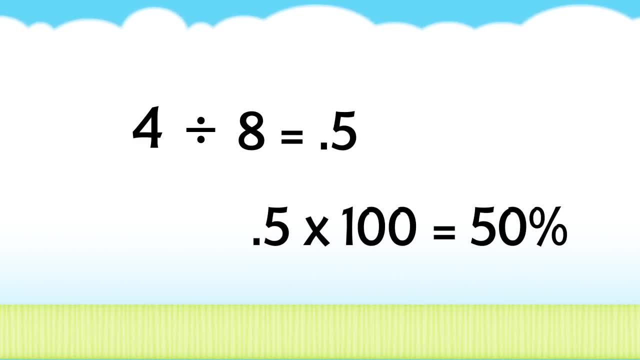 is 50, or 50%. Multiply the decimal by 100, and you've got the percent. Let's try another example. We'll convert the fraction 25, one hundredths, to its equivalent in decimals and then into its equivalent in percents. Divide the numerator 25, by the denominator 100.. The quotient 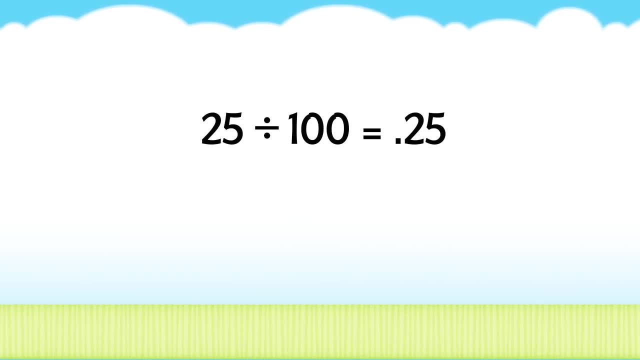 is the decimal 0.25.. Or 25 one hundredths. You see that the fraction 25 one hundredths equals 0.25 of the whole number 1.. To turn the decimal into a percent, multiply it by 100.. 0.25 times 100 equals 25, or 25%. 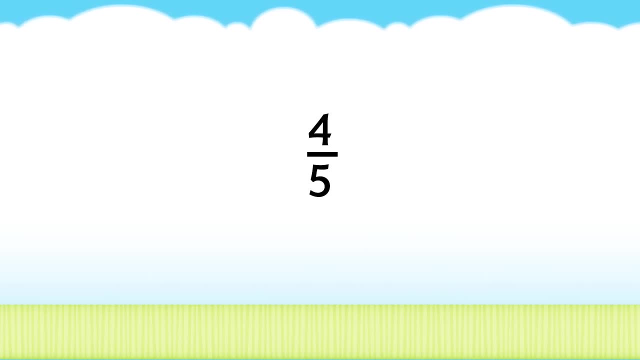 And here's a final illustration: 4 fifths 5, the denominator goes into 4, the numerator 0.8 times. Multiply 0.8 by 100, and your product will be 80.. You can see that 4 fifths is the same as 80%.